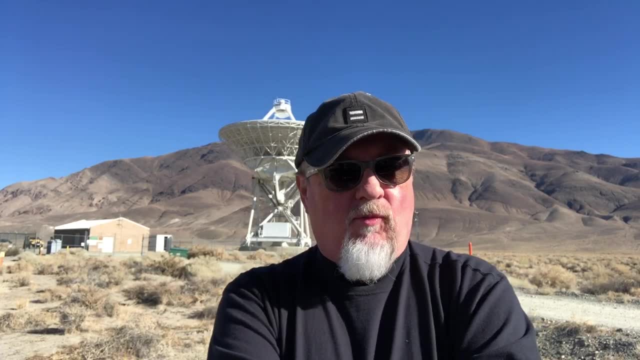 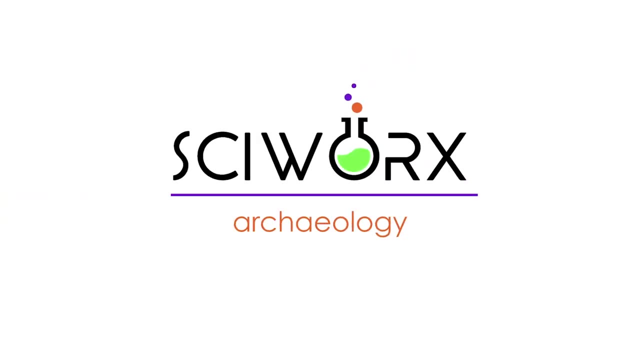 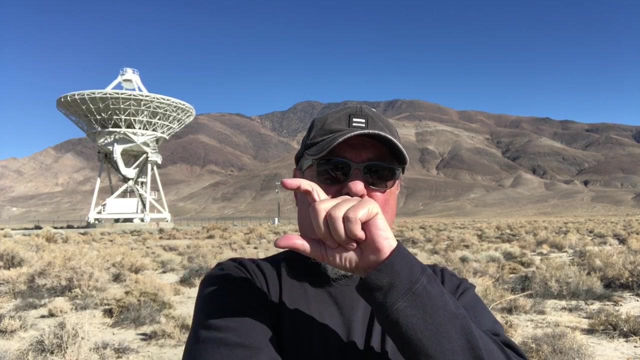 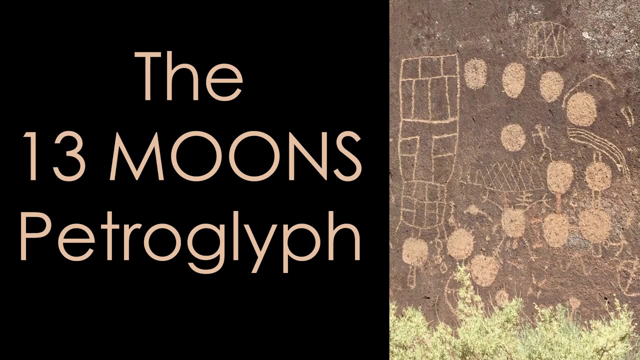 Today we're at the Owens Valley Radio Observatory in wonderful Southern California in the middle of the desert, and we're going to discuss SETI, The search for extraterrestrial intelligence, Mankind. if you've seen my petroglyph videos- 13 Moons and Skyrock- that's filmed north of here in a secret valley- 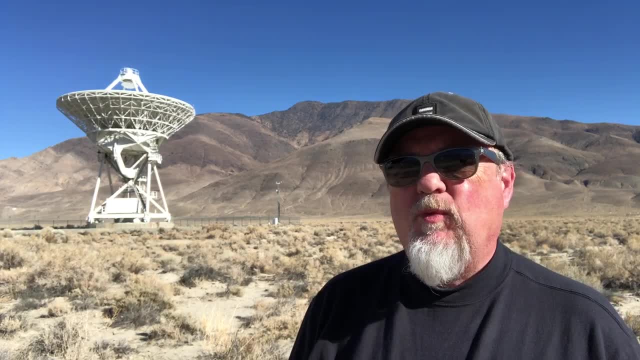 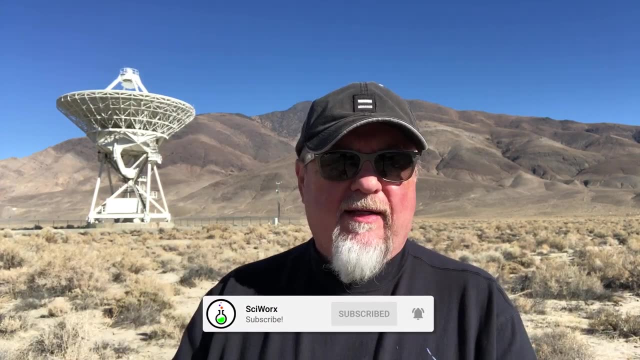 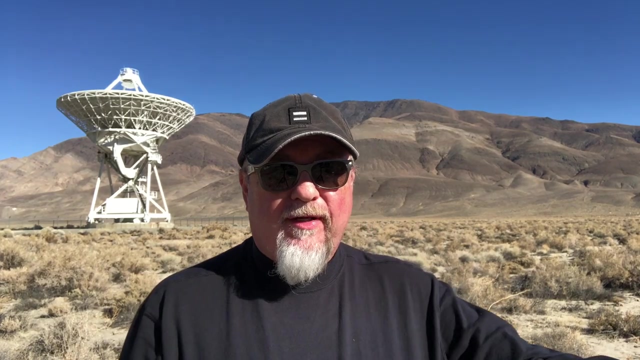 Those petroglyphs were some of man's earliest recognition of the cosmos above. And it just wasn't the Mono people or Native Americans anywhere in North America or South America or Africa or the British Isles or Asia. Humans across the planet have recognized the heavens. 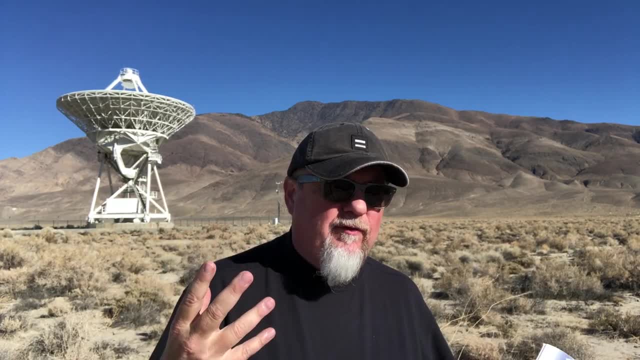 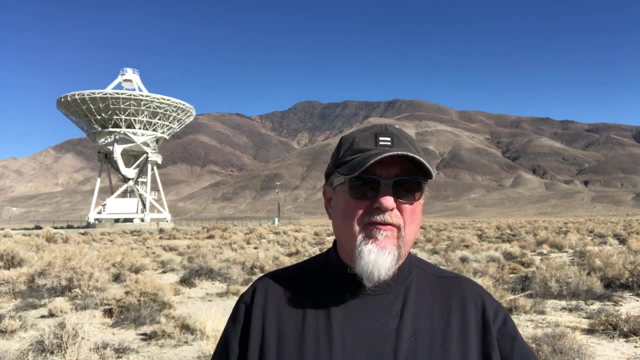 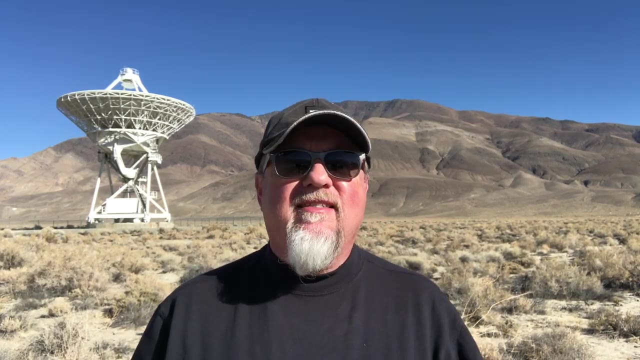 as something magnificent, something wonderful, Something spiritual to behold. We have made movies about it, written novels about it, written love, poetry about it. We have chiseled the stories of the stars into rocks. We have built shrines with tons and tons of solid stone. 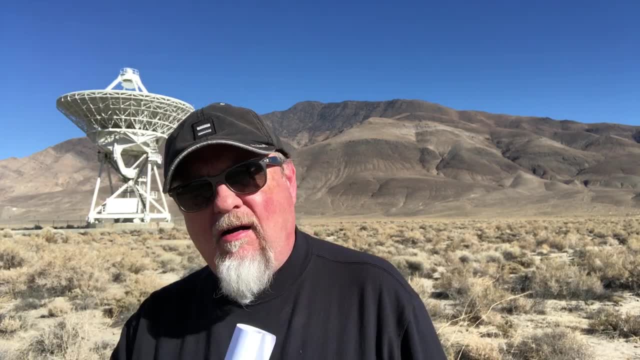 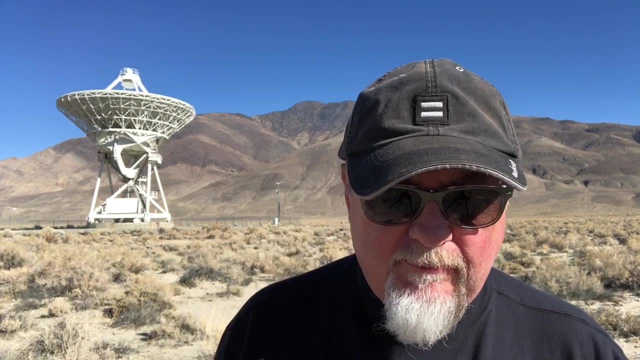 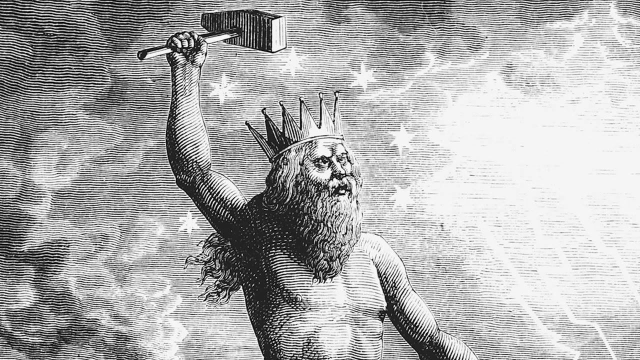 And since all of that time, all of that time, we've always wondered: are we alone? When we started talking, we were talking about a being named Ra, or a being named Thor, or the Coyote God, or the constellation in the sky. 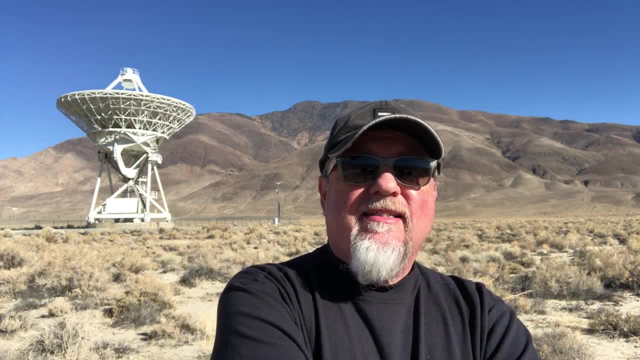 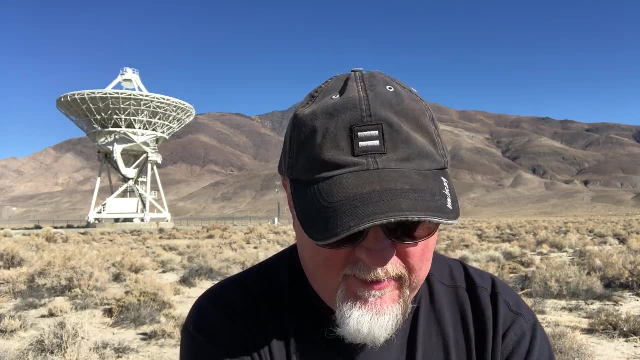 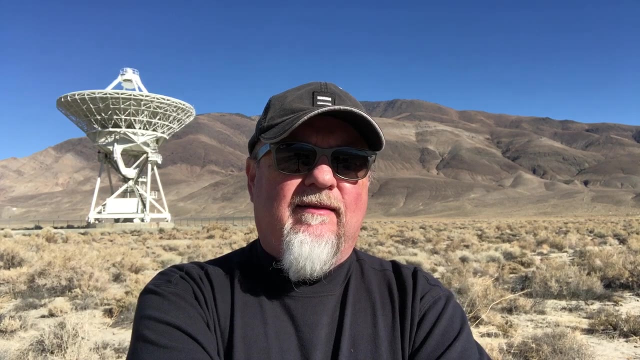 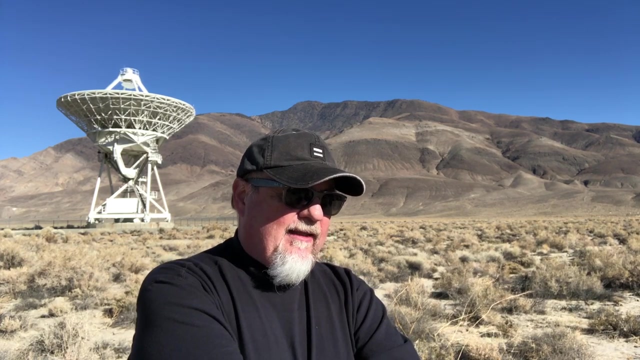 We've always wondered about these beings that live in the sky. Are we alone? Who are they? Why do they look down upon us? There's reams of literature and folklore and storytelling that is fascinating to to absorb, just fascinating to read and watch and listen to, about people other than ourselves. 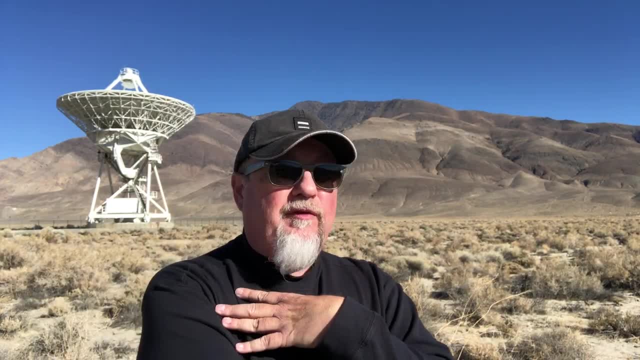 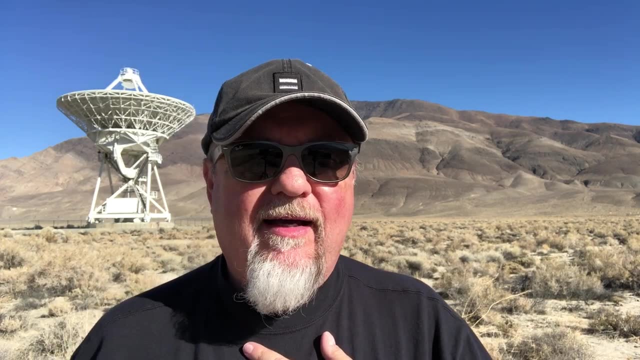 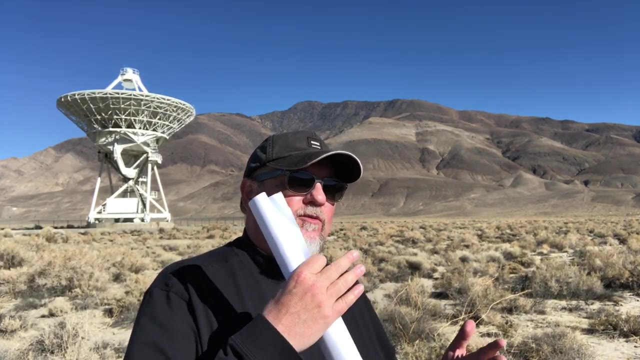 And what's really fascinating is our reflection of those people, the Coyote Gods, that live in the sky. Personally, I think it says more about us than the Coyote Gods up in the sky. But from a scientific point of view, we have to employ first principles: thinking. 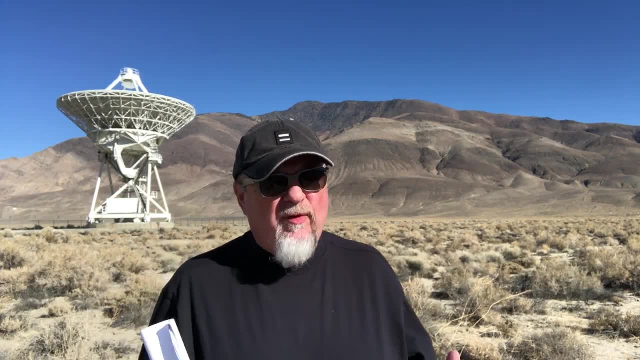 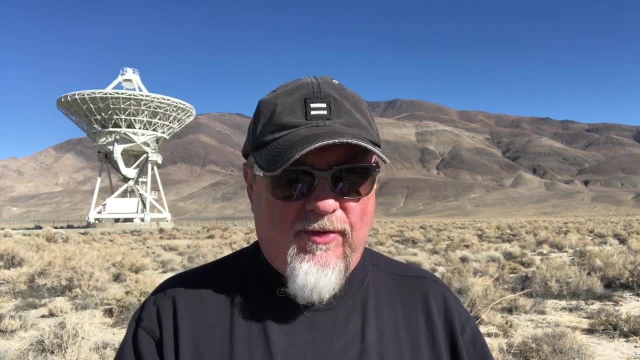 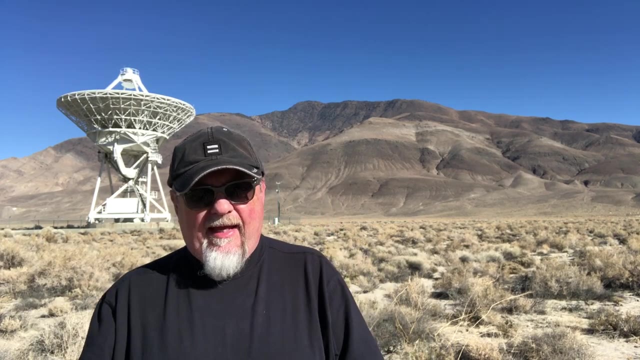 the scientific method to see if we can find real evidence of other civilizations, not of this world, And that's what SETI was about. That's what SETI continue to be about And with every step we take in terms of science, 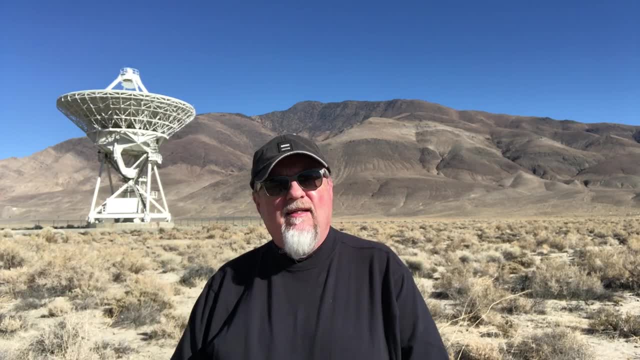 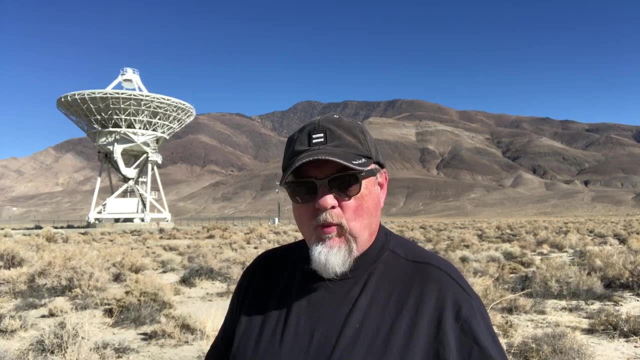 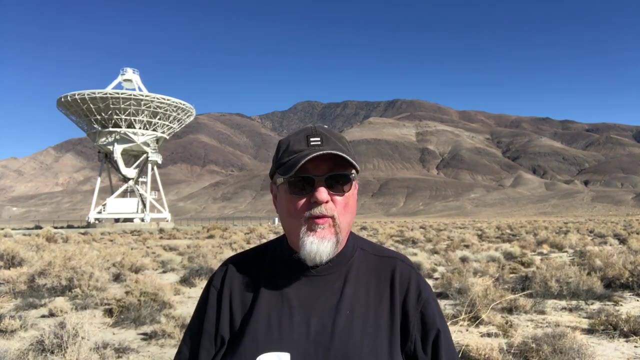 and instruments that we launch into space, places like here at the Owens Valley Radio Tower observatory, with their stair to antennas. we try to answer so many questions, sometimes all at the same time, about what's out there, what does it mean, what do we not know? and we always look for others. there's lots of things we have to. 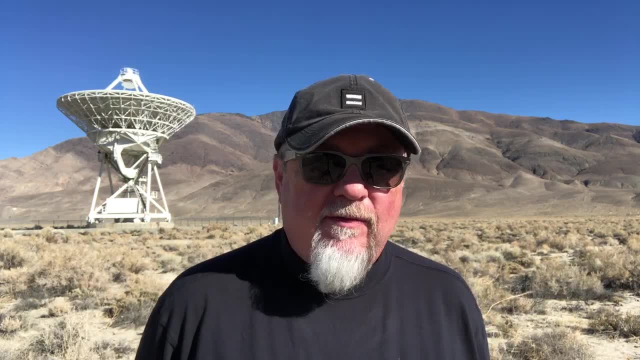 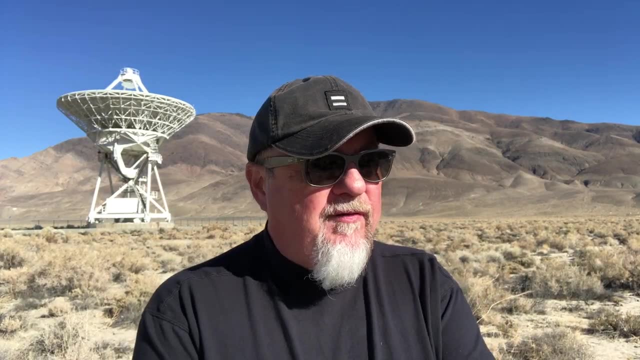 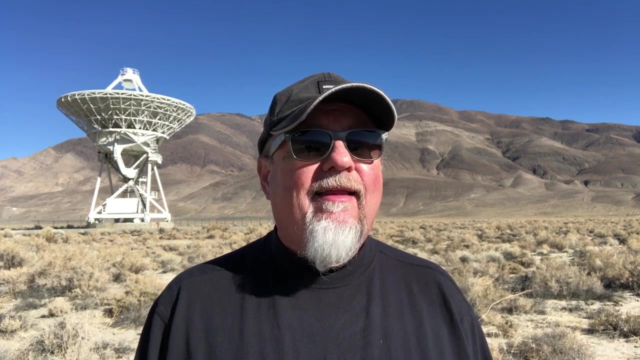 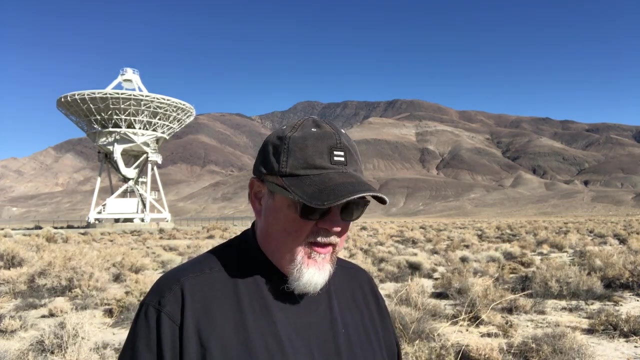 overcome the Fermi paradox. you know that contradiction given name to Enrico Fermi. you know, if there's all these billions of stars and there are all these billions of galaxies and there's all these billions of Earth like planets, well we should be up to our necks. and aliens- where are they? we don't know- with. 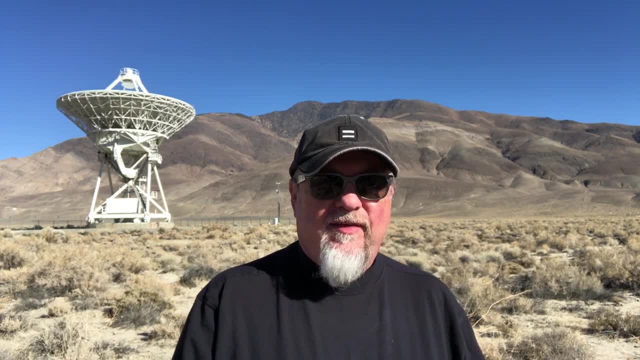 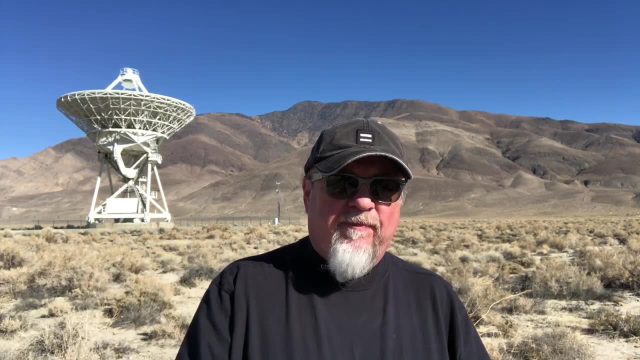 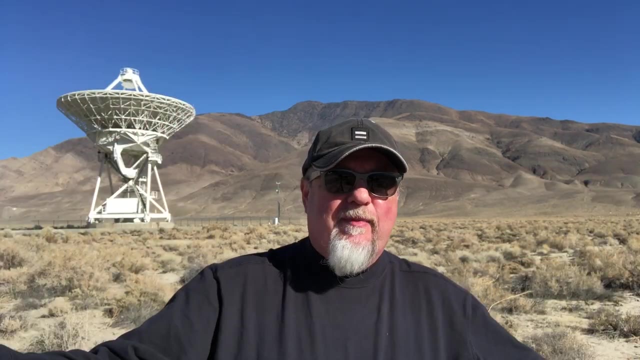 the Drake equation, there's all of these stars, and all of these stars with planets and all of these stars with life, and all of these stars that have life to grow to intelligent species, and all these intelligent species that develop a technology, all of these species that actually broadcast electromagnetic energy into universe. 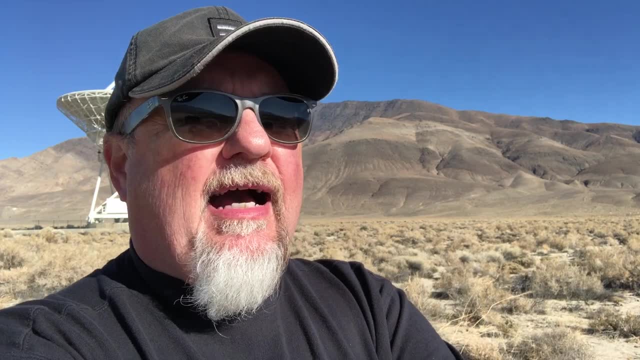 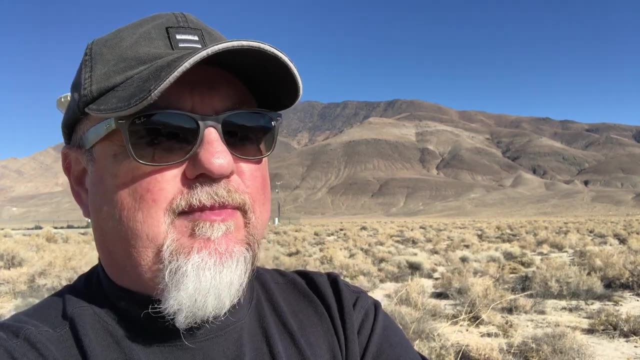 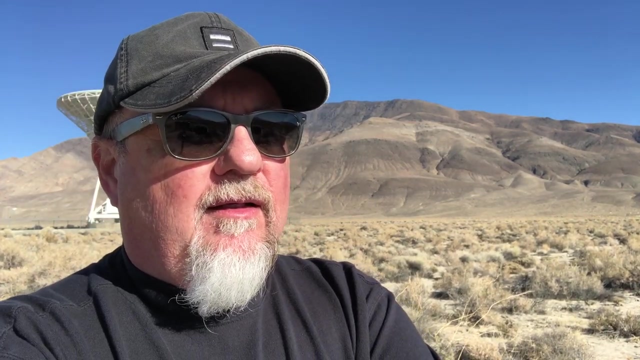 where are they sidebar? I'm not discounting the recent revelations from the office of naval intelligence saying that the United States government is in possession of a craft, not as of this earth or the tic-tac videos. like dr Sagan said, extraordinary claims require extraordinary evidence. a memo from the 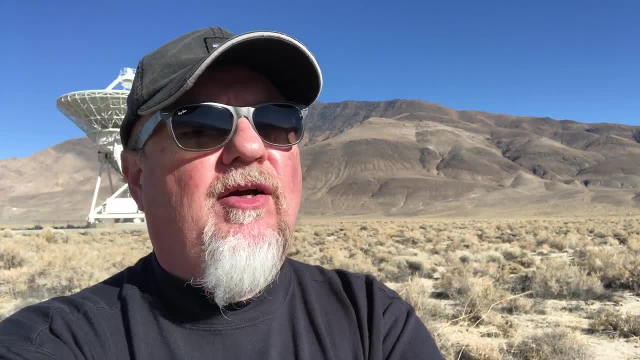 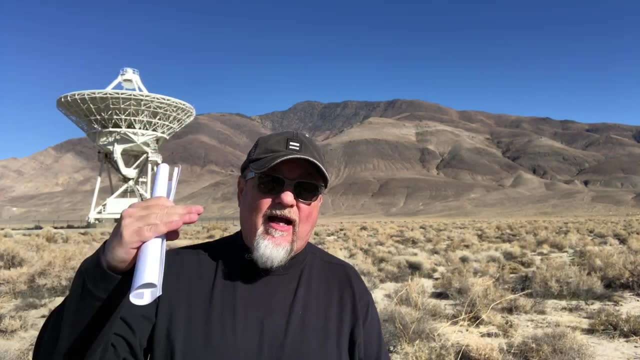 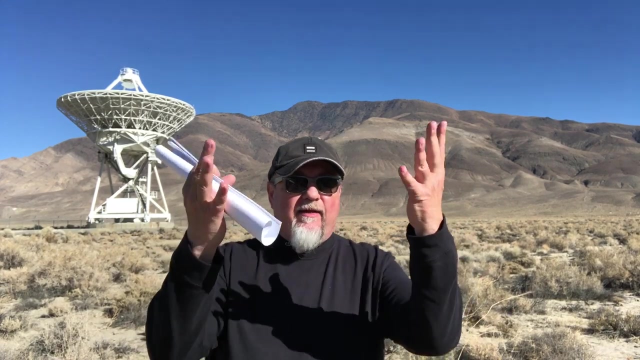 office of naval intelligence isn't that? we got to look harder. we have a scientist, we have a higher level of credulity. we have to maintain. we have higher hurdles we have to jump and we have to be completely transparent. we got to throw all of our data out on the table. what do you guys think? what do you? 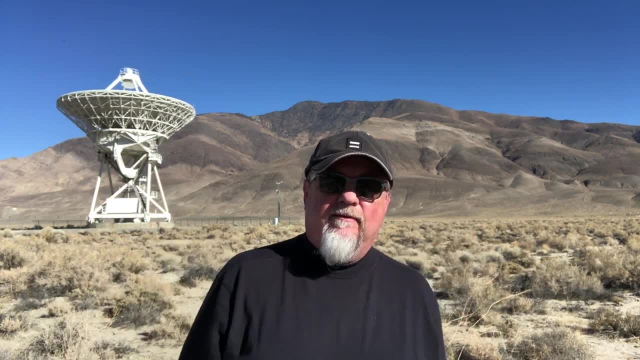 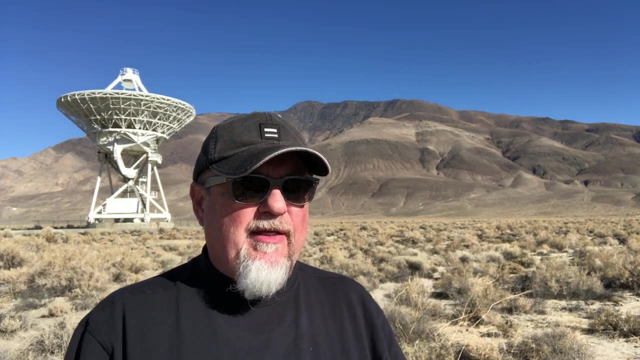 what do you guys over there think? tell me, what do you make of the data? that's how science is done. and said he's a tough one. now said he is one of mankind's most remarkable searches. we nothing could be more consequential to our own daily lives with the 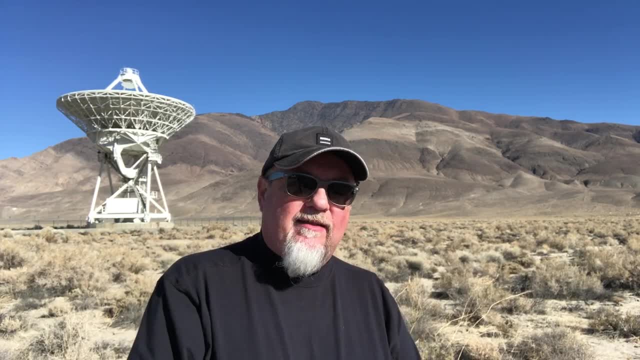 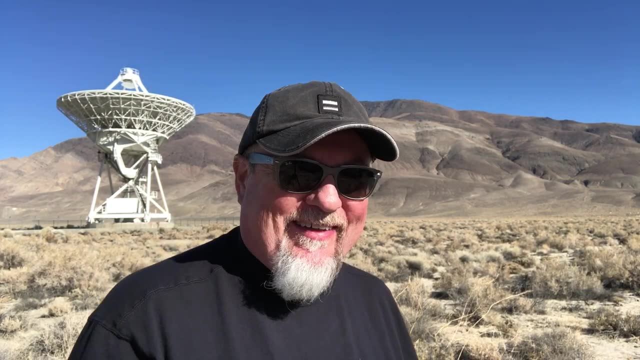 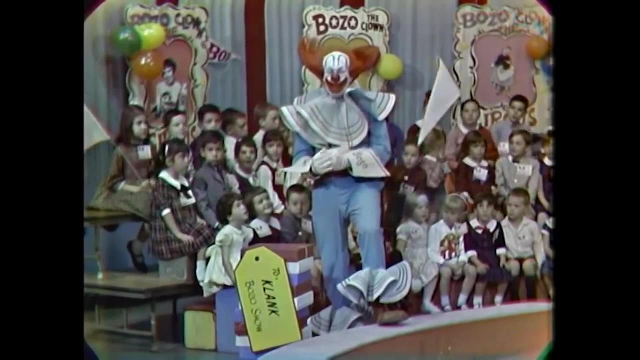 knowledge that there are civilizations out there that actually had worse television programs than we do. I mean, wouldn't that be of some comfort to you, right? I mean, have you seen some of the stuff that came out of the seventies? wow, because I was kind of excited. 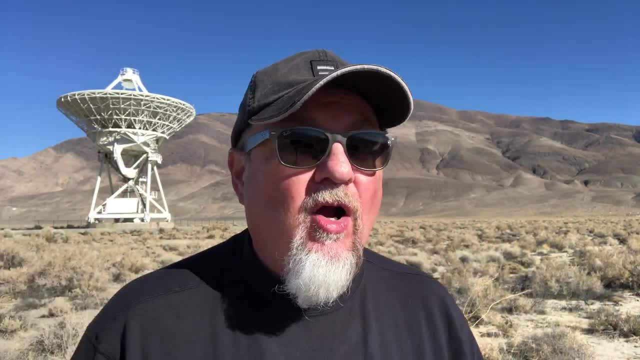 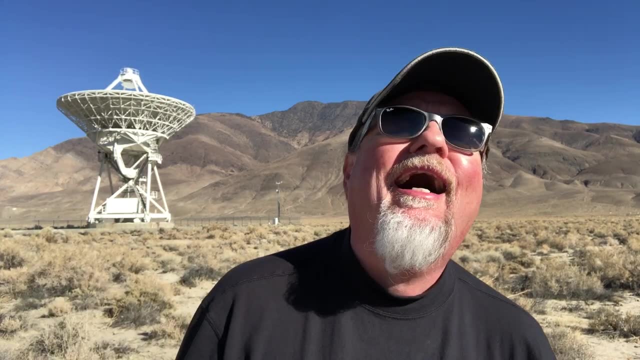 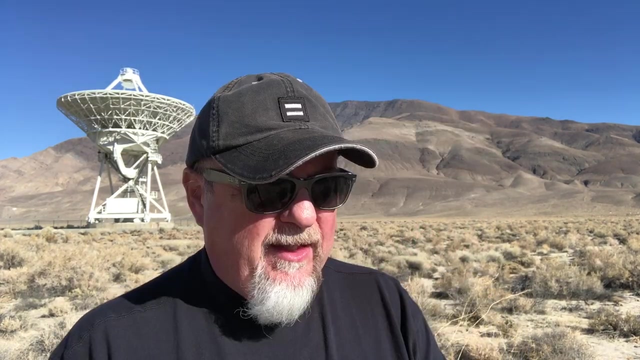 why somebody even bothers to put that on YouTube. I don't know. why are there subreddits for these crappy TV shows and then with hundreds of users, why I don't understand. so maybe give us hope that there's somebody out there in the universe has crappier TV shows in us. 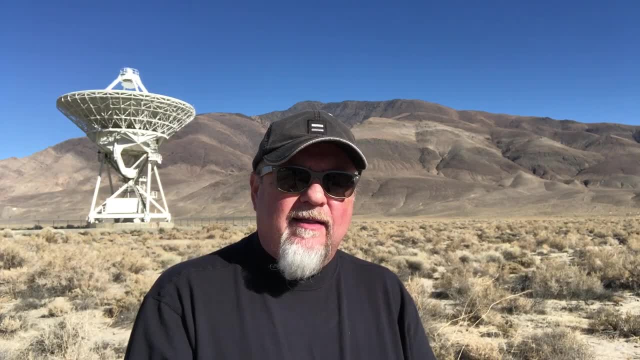 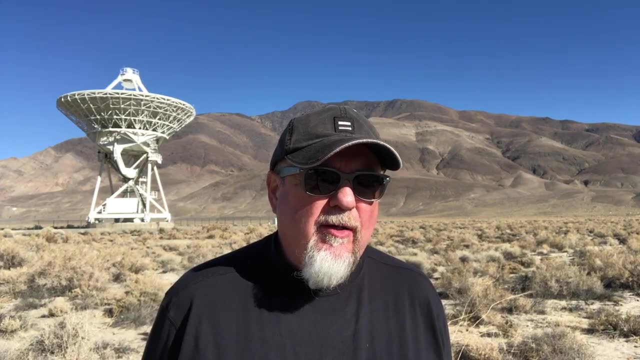 you know there's there. there's a effort underway by citizen scientists and scientists and just people around the world trying to get America to rebuild Arecibo. Arecibo put out the most important message the SETI community has ever done and that was the Arecibo message. 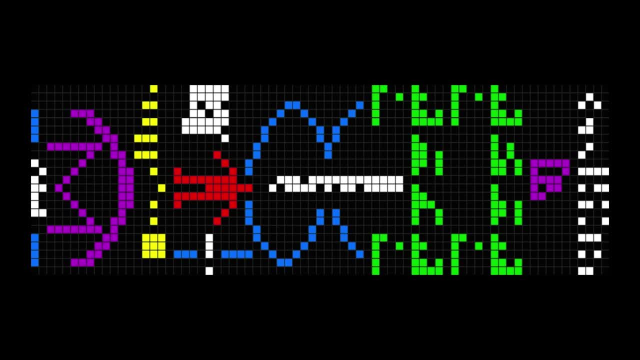 as you can see here, it was a series of blocks. it was a blocked Matrix showing all about us, how we send signals, the science of parabolas, pictures of ourselves, where we live. we have a double helix, or organic, uh, biology, and we send it out with those. 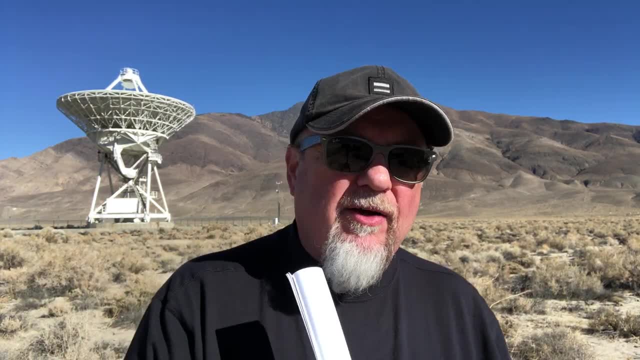 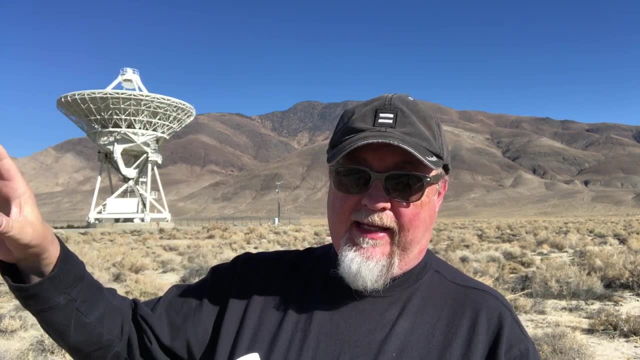 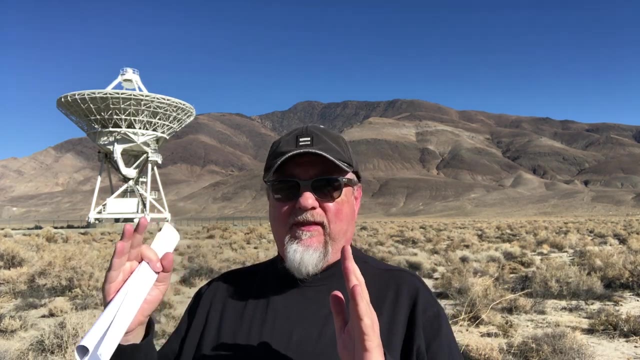 Arcebo. we have not heard back from since. in the very shortest amount of time it would take to get to some other planet where we think there may be a planet, it's still going to take dozens and dozens and dozens of decades, traveling at the speed of light. 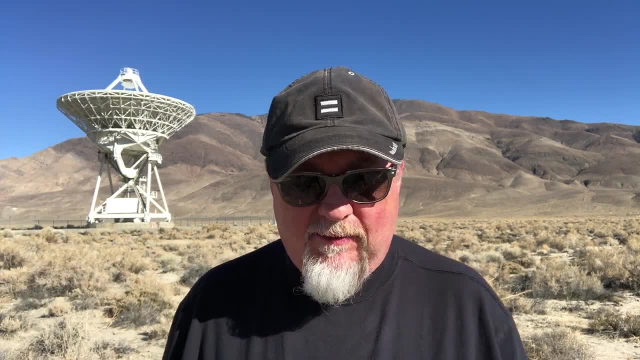 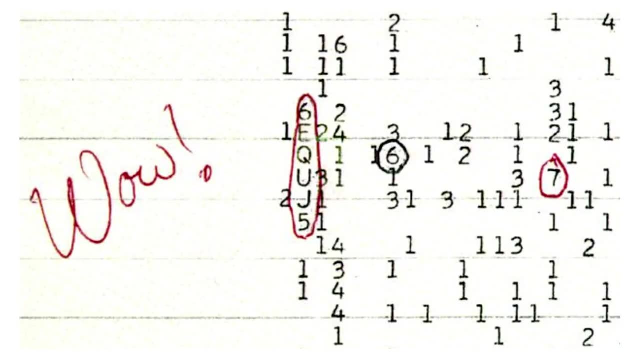 for them to even receive it, if they are there at all, we just don't know. there has been a lot of positive work done for the SETI project. there's the wow signal. you know that came from the Ohio State SETI program, something we have never seen before. we've never seen, since. we don't know what it means. was it really a fast radio burst? we don't know, nor do we have the funding to really find out. UC Berkeley started the SETI at home project. it was wildly successful, so much so they've got more data than they can look at these days they had.